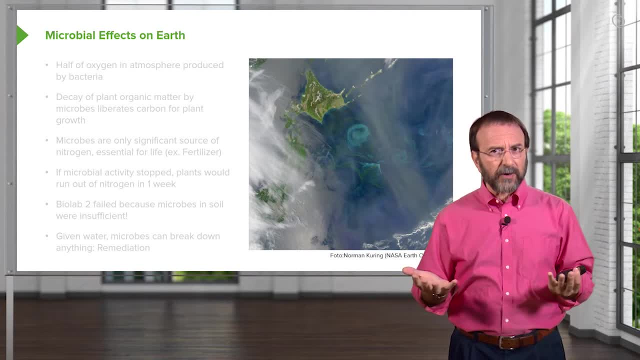 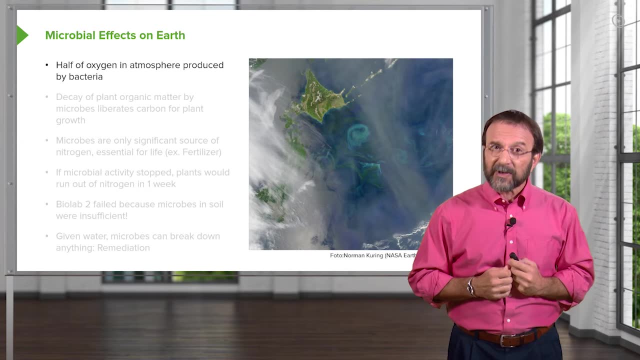 can use. Microbes have shaped our earth in many different ways. Half of the oxygen that you are breathing today is produced by bacteria. Plants decay because of the microbes that are present in soil. If it weren't for the microbes, the plants would never decay, and 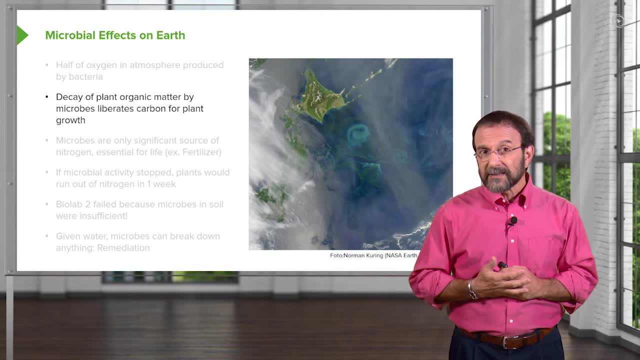 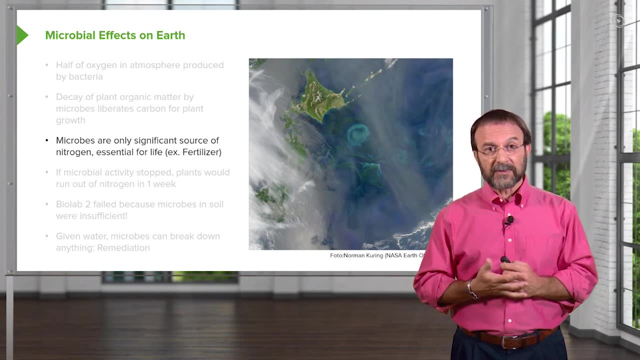 that would bring about carbon emissions. Carbon would never be recycled. Microbes are the only significant source of nitrogen on the earth. This is essential for plants to grow, and microbes take the nitrogen gas from the atmosphere and convert it to chemicals that plants can use. Humans know how to do this. We make fertilizer, for example- but microbes 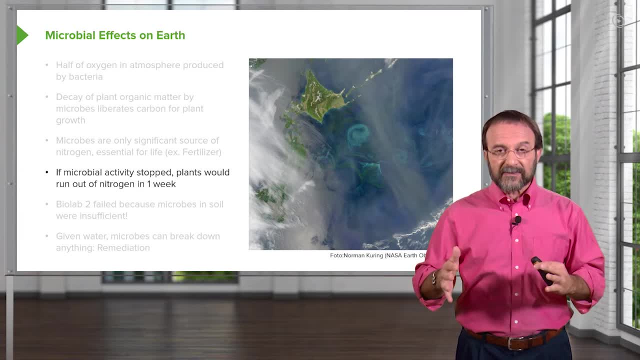 are essential for plants to grow. If microbial activity on the planet were stopped, the plants would run out of nitrogen in a week And we wouldn't be able to make enough fertilizer to make up the difference. You may be aware of a scientific experiment done a number of years ago. 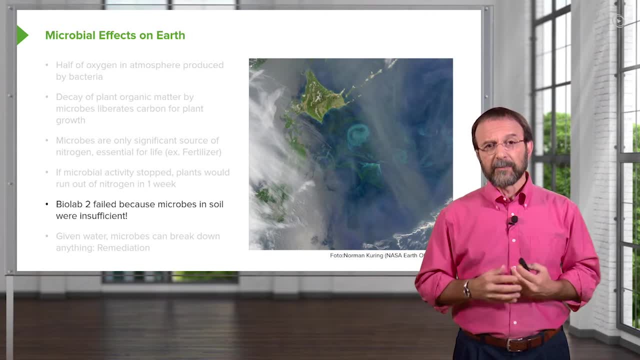 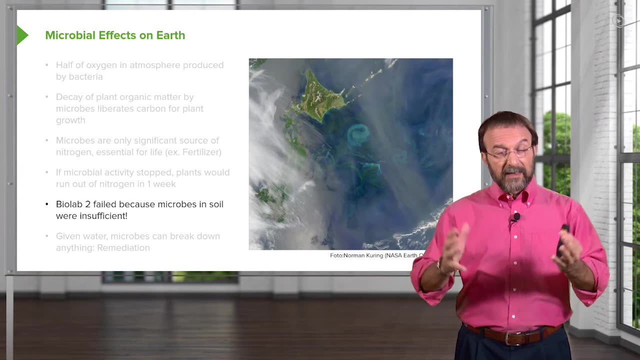 called BioLab 2.. This was a lab built in the desert of Arizona. A few humans were put into this, plants were put into this, and the idea was that the humans would be self-sufficient. They would grow all of the food that they would need and dispose of it as well. 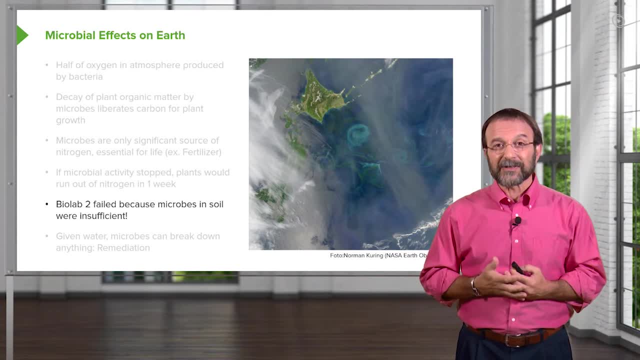 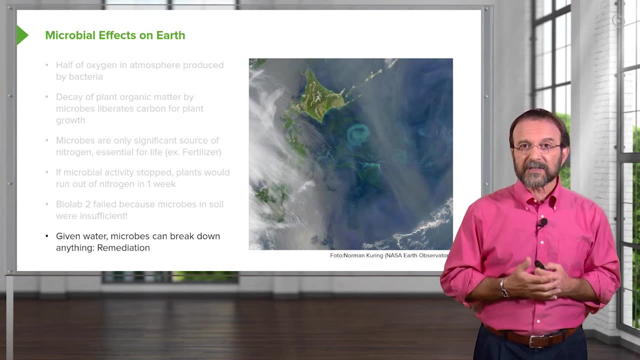 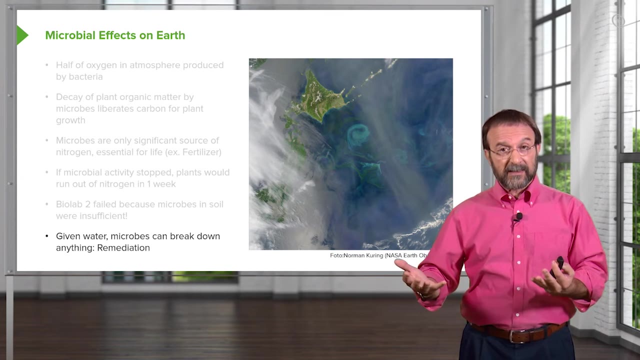 Well, this experiment failed because we didn't put the right bacteria in the soil to generate the compounds that the humans needed to survive. So, given water, microbes can break down anything And we use this for remediation. So, for example, if there is an oil spill in the ocean due to a tanker breaking or 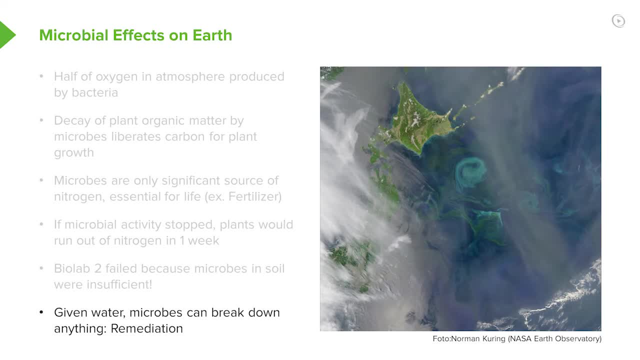 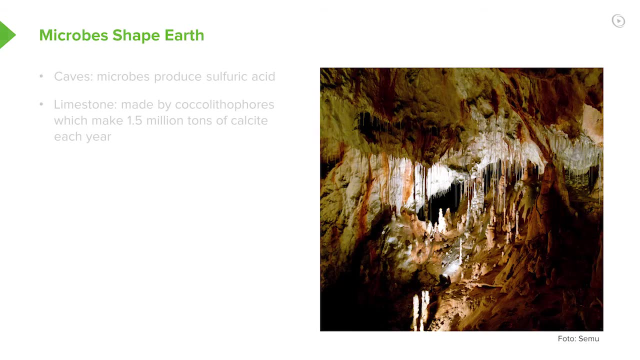 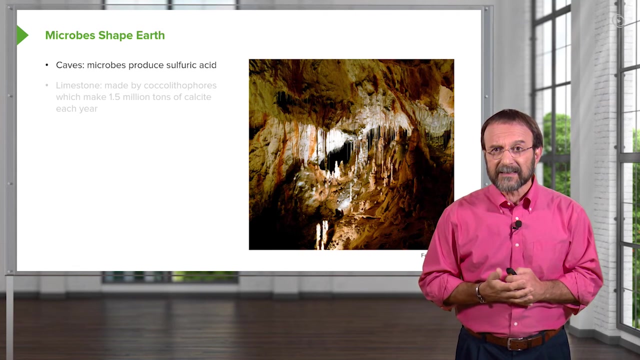 a broken pipeline, we can add bacteria, which will then degrade the oil. Microbes also shape the physical earth that we live on, The caves that you are familiar with, with the open caverns and the stalactites and stalagmites growing from the walls. 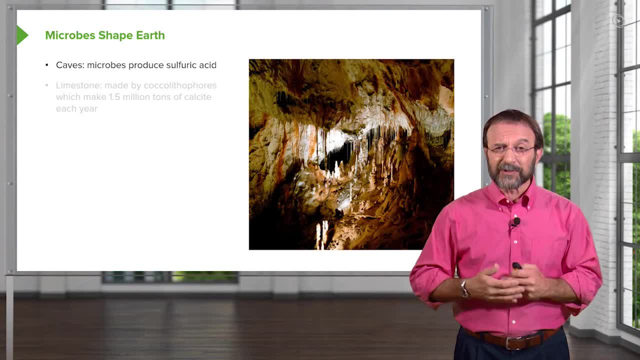 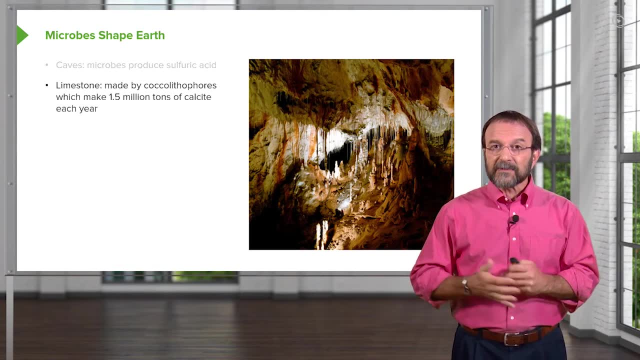 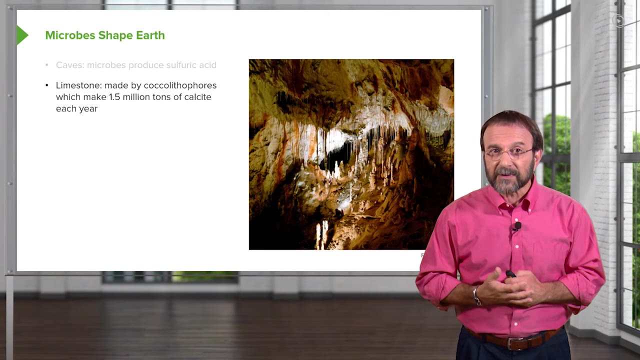 these are produced by microbial activity. Microbes actually produce sulfuric acid, which plays a role in eroding away the stone. The limestone that makes up so many caves is actually a microbial product. A microbe called a coccolithophore makes about.